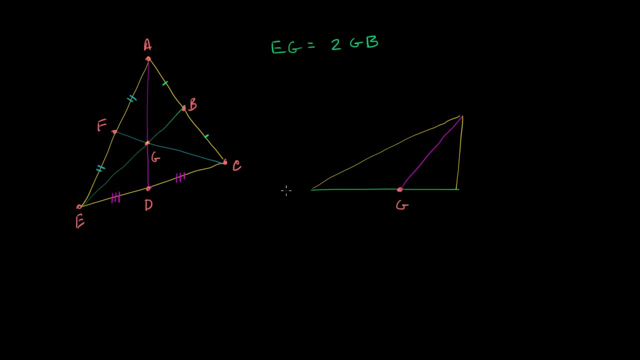 Let me draw it a little bit neater than that. We have that line going to A, And then we have this blue line going to F. right over here We have this blue line going to F, And let me label all the points. 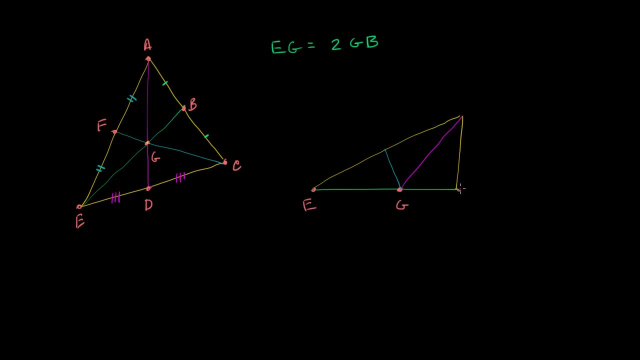 Go back to the orange color. So this is going to be E, This is going to be B, This is going to be A, This is going to be F. right over here, And just to make sure we have all the same markings. 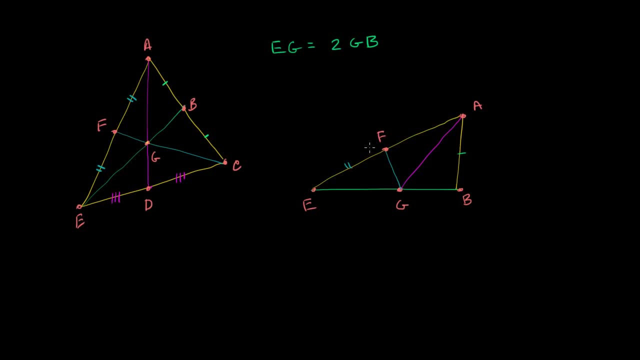 that little marking. there is that marking. These two markings are on this side, right over there, And the whole way that I'm going to prove that EG is twice as long as GB is just refer to the result that we did. I think. a couple of videos. 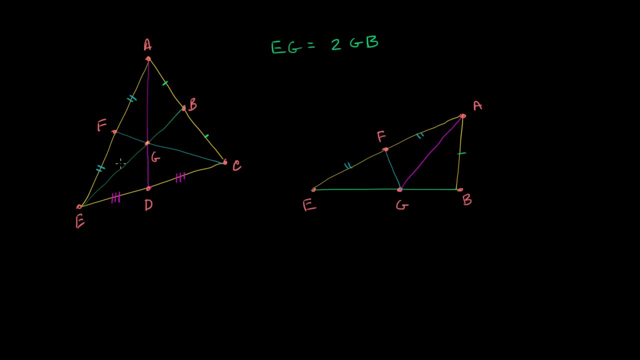 ago that the medians divide this triangle into six smaller triangles that all have equals. They all have equal area. So another way to think about it is each of these three smaller triangles have equal area. These are three of the total of six smaller triangles. 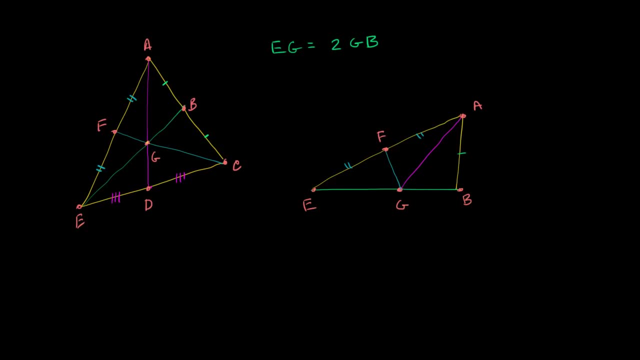 So these three all have equal area. So let's think about this triangle right over here. Let's think about this triangle triangle AGB. This is triangle AGB right over there. Those are the same triangles. And let's compare that to triangle EAG right over here. 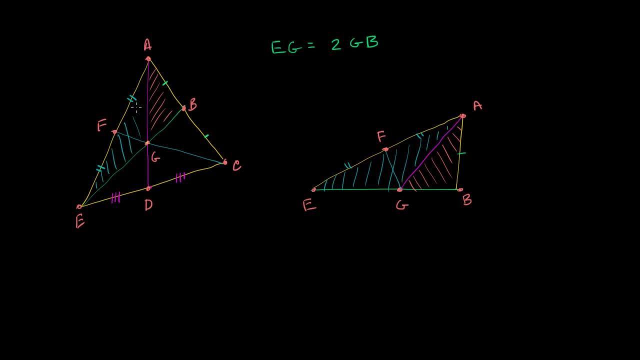 Let's compare it to this triangle, which is this triangle, This triangle right over here on the original drawing. Now they both have the exact same height. If you view EG as their base- or, I guess, their shared base- they don't have the exact same base. 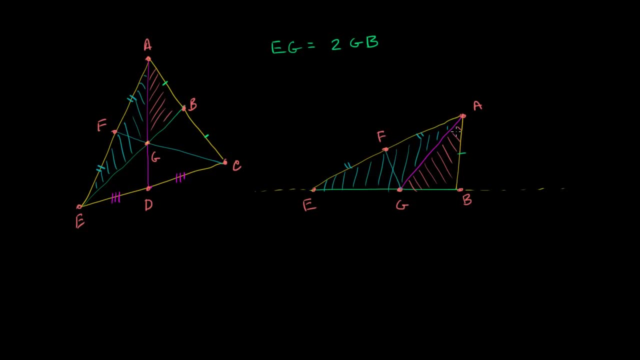 The smaller orange triangle has GB as its base. The larger blue triangle has EG as its base, But they definitely both have the same height or altitude when you draw it this way. So their height in both cases is this right over here. 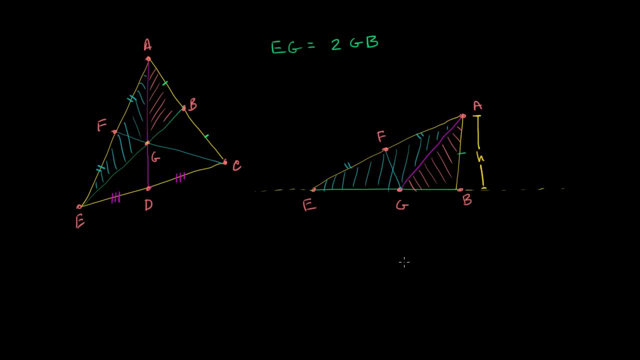 Now the other thing that we do know is that this blue triangle, EAG, has twice the area of the orange triangle. How do we know that? Because it's got two of these triangles in it. So one way to think about it is: if this orange triangle 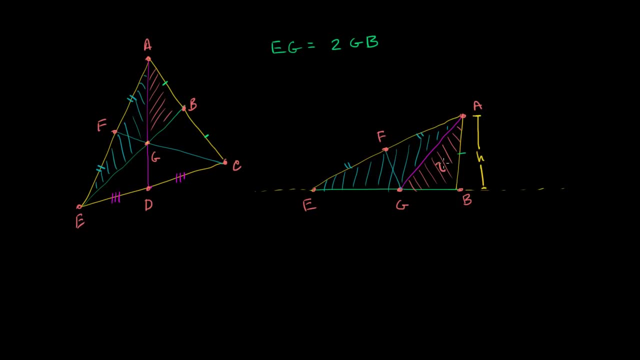 has area x, which I'm going to call it A. Well, I already used A, So I'm going to call it area x. Then each of these blue triangles have area x. Or you could say: this entire blue, this entire blue region, has area 2x. 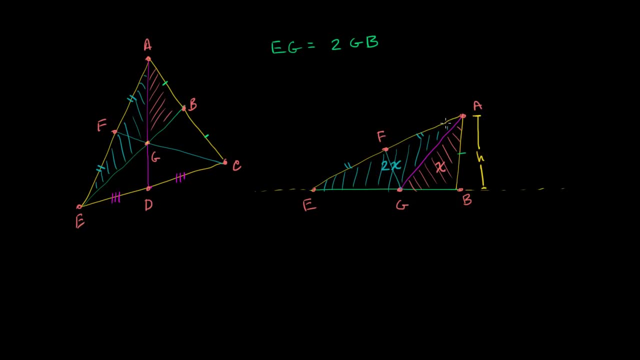 So if you look at this blue triangle right over here, we know that 1 half times base times height is equal to area, So we get 1 half. The base is EG. I'll do that in the green color: 1 half EG times height, times this yellow height. 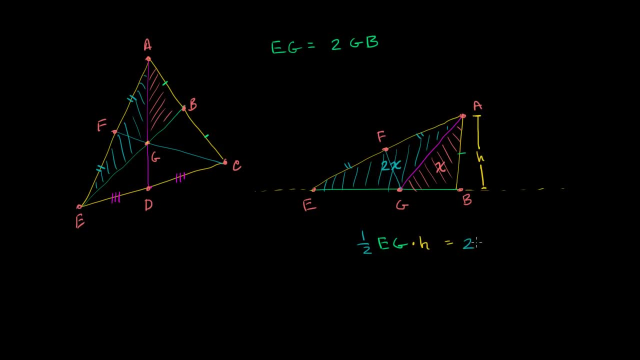 is going to be equal to 2x. 2x is going to be equal to 2x. I'm just applying the formula for area of a triangle: 1 half base times height is equal to area. This is our area. 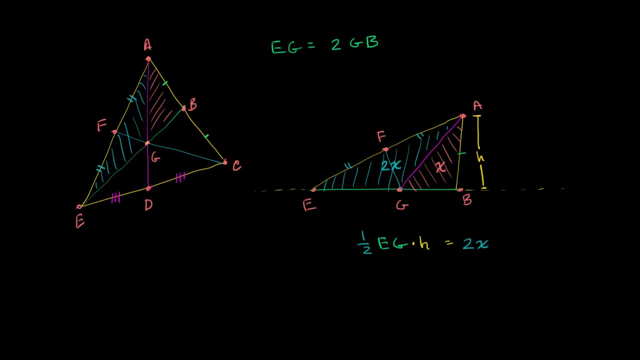 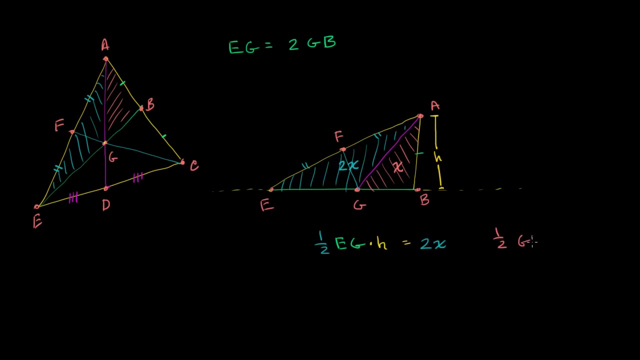 Now let's do the same thing for this orange triangle: 1 half. let me scroll over a little bit to the right. We have 1 half GB times the yellow height times height is going to be equal to x. Well, we can substitute. 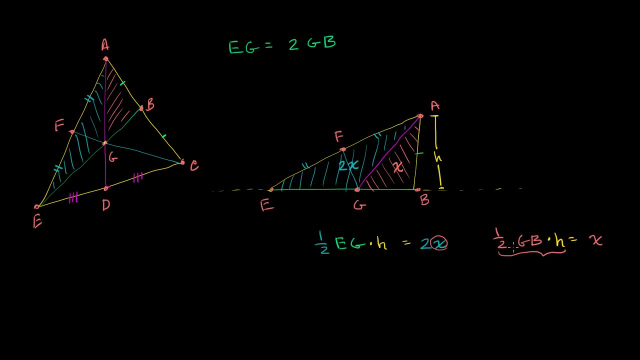 If this is equal to x, we can place this entire expression right over here for x. So let's do that. We get 1 half And you might already see where this is going, but I won't skip any steps here. We get 1 half times EG times H is equal to 2 times H. 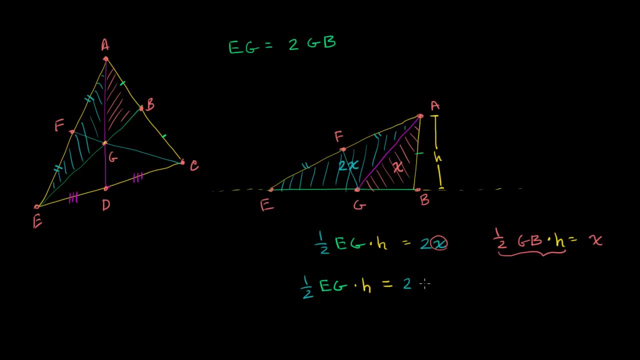 But instead of x I'm going to write this here. It's equal to 2 times 1, half, times GB, times this length, times the base of the smaller triangle, times H. And now we can just simplify this. We have 2 times 1. half is just going to be 1.. 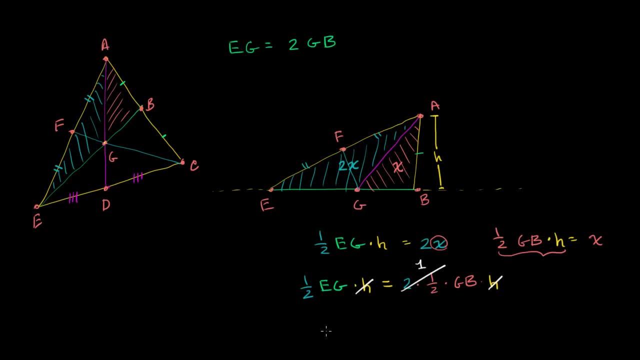 You can divide both sides by H And we are left with: 1 half EG is equal to GB. Or we could write EG. Let me do it in the same color, since I've gone this far with the same colors. So we can write: 1 half EG is equal to GB.